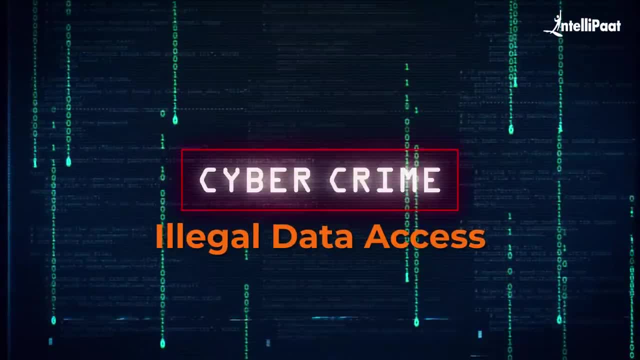 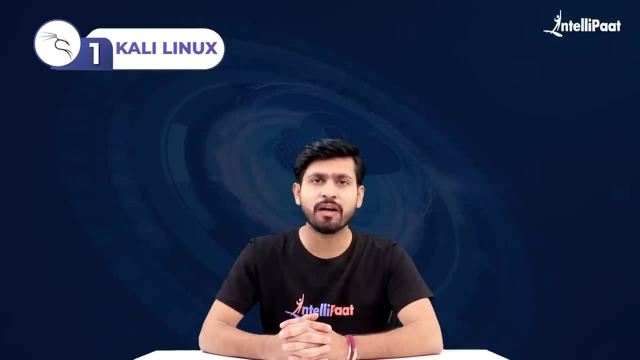 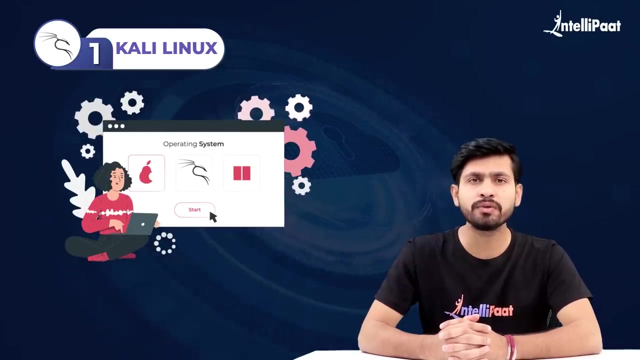 It is employed in order to prevent illegal data access, cyber attacks and identity theft. So the first tool that we are going to study about is Kali Linux. Kali Linux is among the most common tools used in cyber security. This operating system consists of a range of tools that are used in security, auditing, network and system scanning for vulnerabilities. 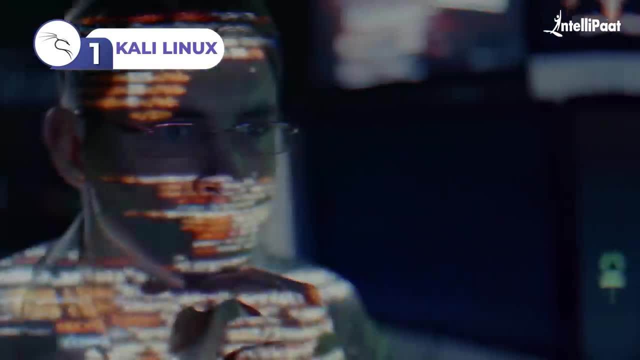 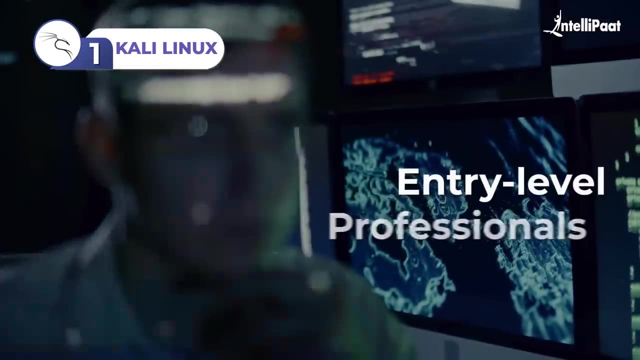 One of the main advantages of this platform is that cyber security expert with different levels of understanding can use it, Making it an ideal choice for even an entry level professional. The second tool that we are going to discuss is Metasploit. Metasploit has an excellent collection. 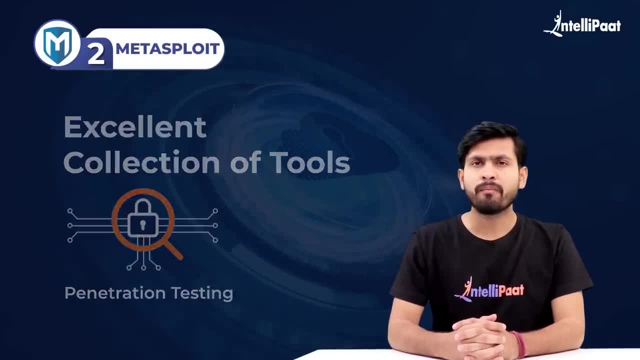 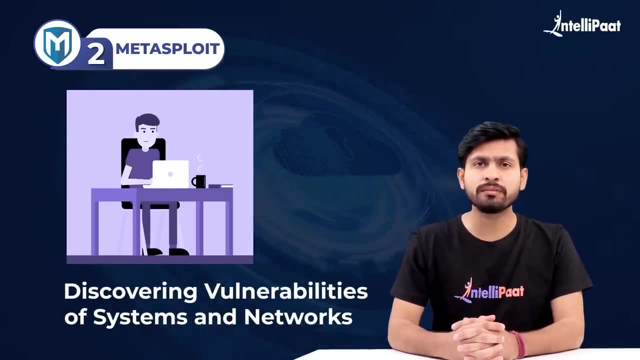 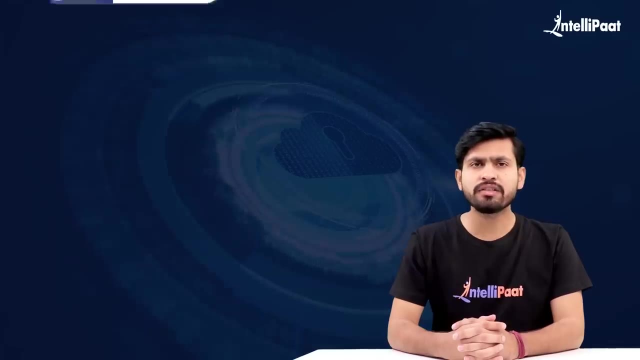 Of tools that are perfect for penetration. testing Professionals often use it to meet a wide range of security objectives, Such as discovering vulnerabilities of system and networks, Designing strategies to improve the company's cyber security defenses, and many more. Let's discuss the third tool, that is, Johnny Ripper. 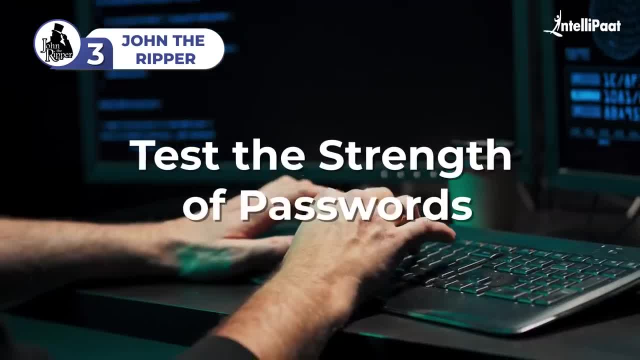 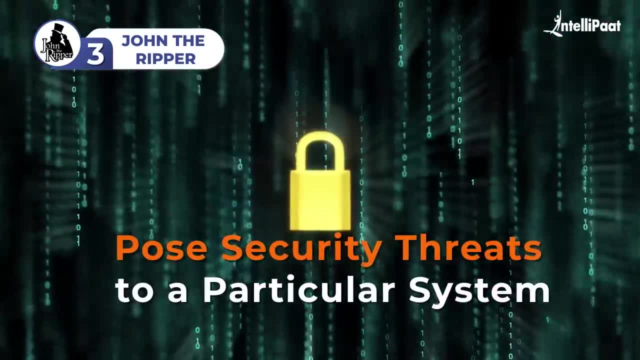 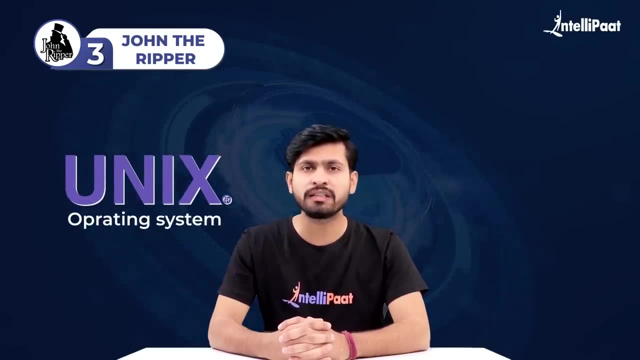 Security experts use Johnny Ripper to test the strength of passwords It designs. helps in exposing weak passwords that cause security threats. It can be used to hack into a particular system. In the beginning it was only designed for the Unix platform, but the new version allow it to work on the other operating systems as well, such as DOS, Windows, OpenVM and etc. 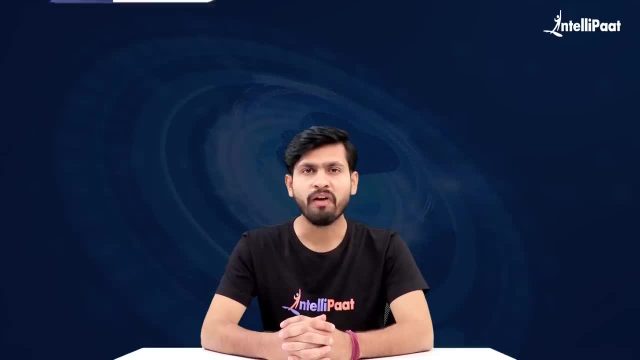 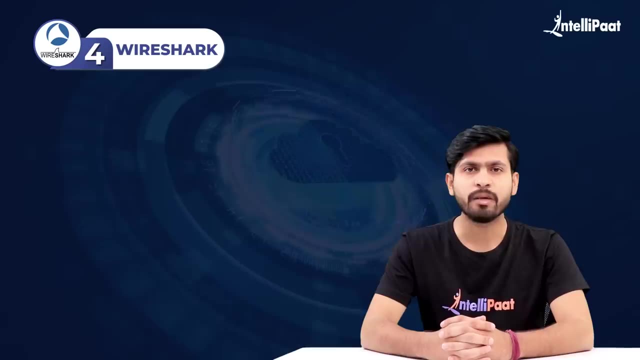